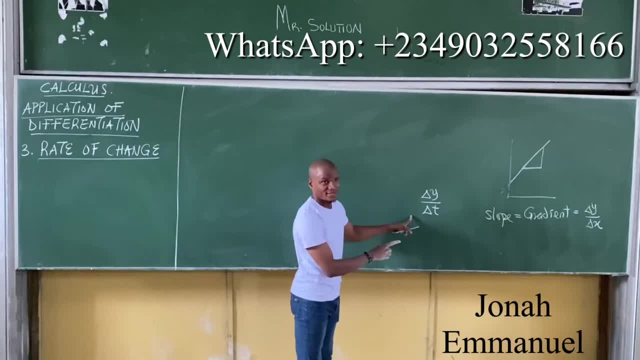 This will be called the rate of change of y. That's it. So hence, if you say the rate of change of area, that becomes what Change in area? all the water change in time, That's all. If you say rate of change of radius, 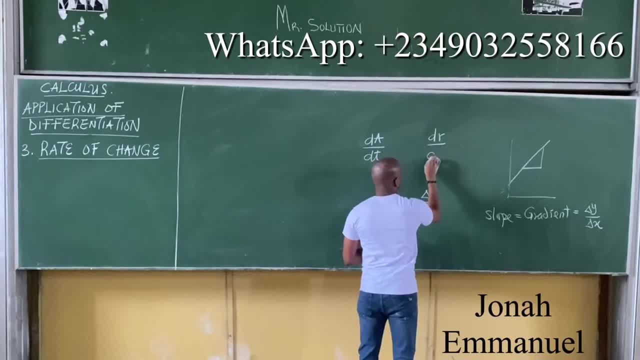 becomes what? Change in radius, all the water change in time. One last thought: If you say rate of change of, let's say, height, it becomes what? All over depth change in height. All over depth change in height. 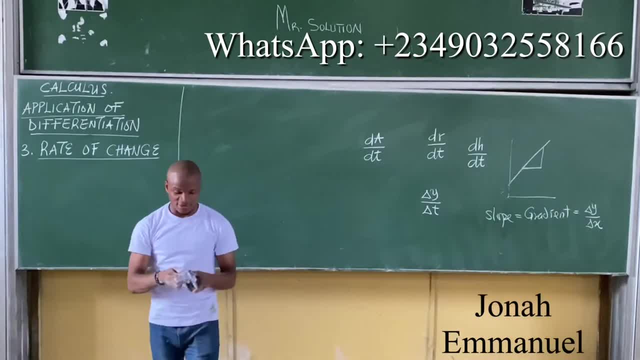 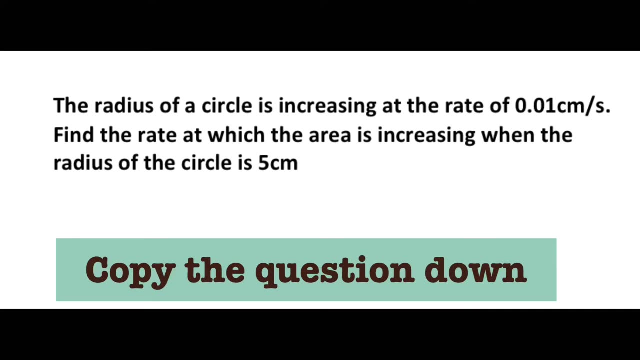 It's just this simple, That's all. It's just this simple, That's all. Take that with you. Take that with you. Sample problem, please Question one. Sample problem, question one: The radius of the circle is increasing. 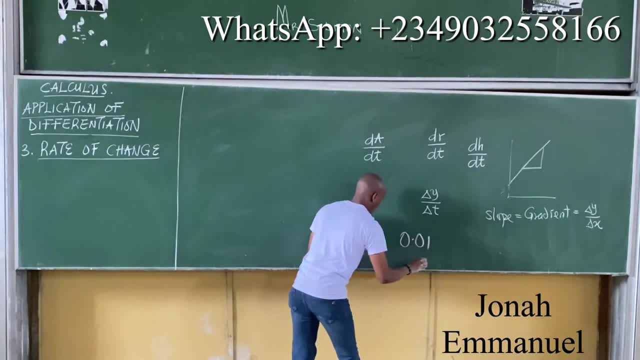 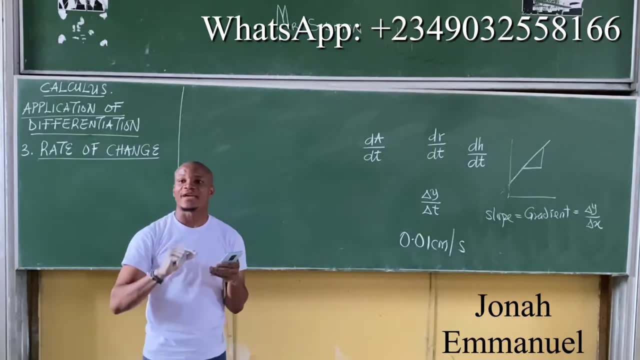 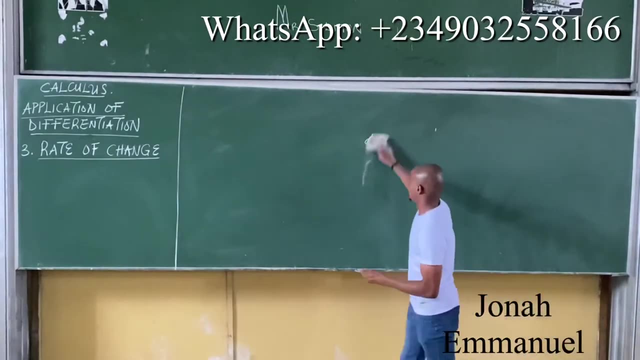 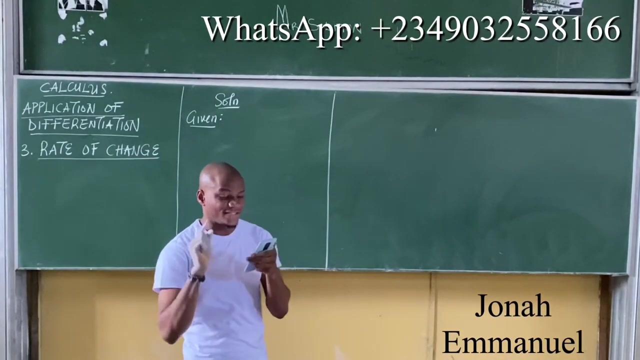 at the rate of 0.01 cm per circle, Find the rate at which the area is increasing. when the radius of the circle is 5 cm, Let's check what we are getting there, Given, given, they said, the radius of the circle. 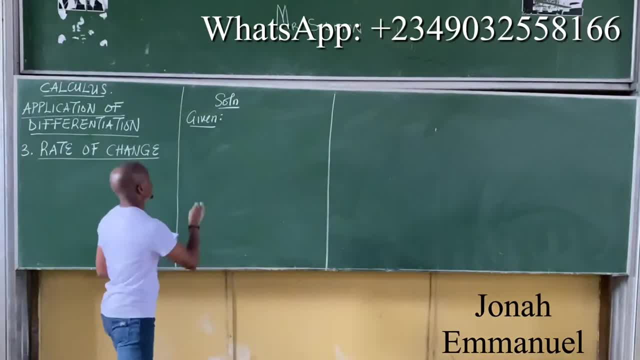 is increasing at the rate number one. Note that the radius is increasing at the rate, So the cost over there, the angle, over there the Z, the rate is increasing. At what rate? there It's equal to what? 0.01 cm per second. 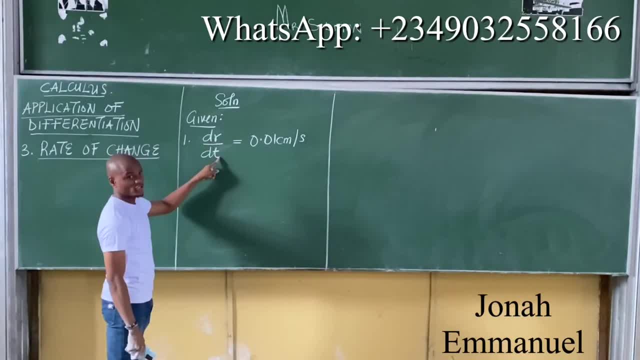 It makes sense. Radius in centimeters, time in seconds: So it makes sense. Let me check this part please. Some will say increasing, some will say decreasing. So what's different When it is increasing? it's what there. 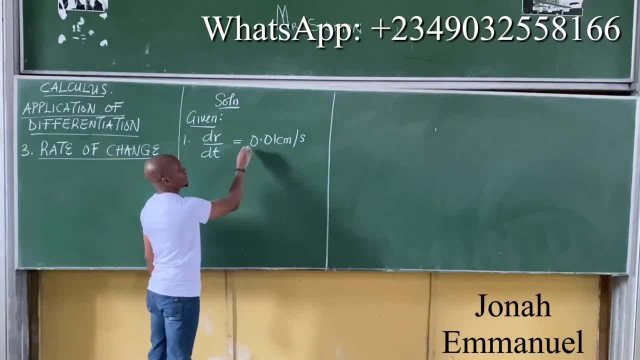 Positive. If this one is increasing what's over there, Negative. So, as you may see, this one here is decreasing. I'll put negative there, That's for sure. So increasing at this rate. okay Number, they said. find the rate at which what there. 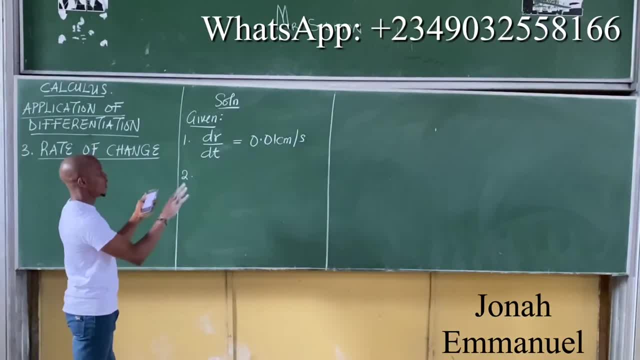 area is what? Increasing, Increasing. What will be your piece in there? For area, what do you have? A, The A over what? The Z? The Z is equal to what there, Unknown, They find the rate at which the area is increasing. 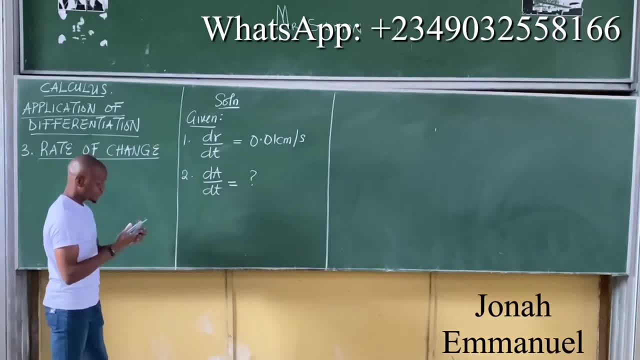 So the A over the Z is unknown, They said: when the rate of the Z is what? 5 cm? Number three radius. radius r is equal to 5 cm. So we have this. Let me chip in here please. 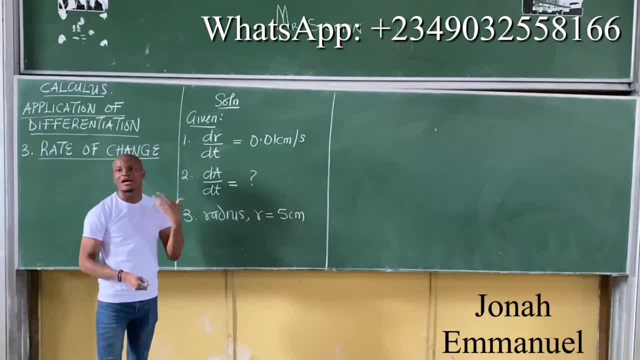 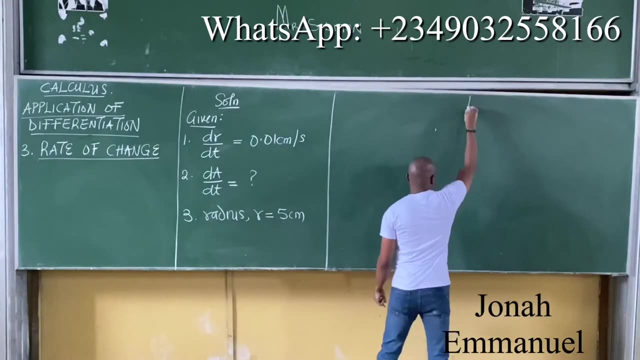 The major problem here is if you cannot remember your formula correctly. That's the problem here. If you cannot remember your formula correctly, For instance, dimension area, dimension radius, Please check in this question which shape or which figure is being considered. 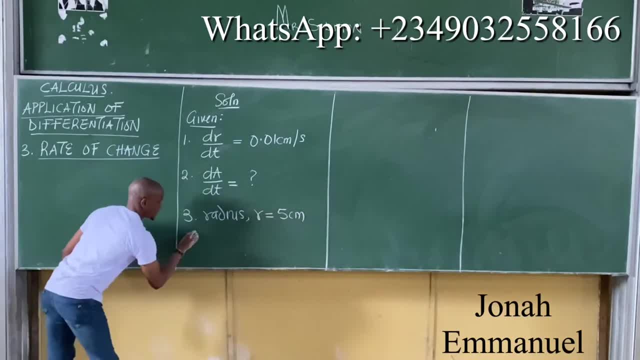 Circle, Circle, All right. So for circle, let's have a space For circle. For circle, Let's have a space Circle. What's the area of the circle? 5.. 5 and the square. 5 and the square. 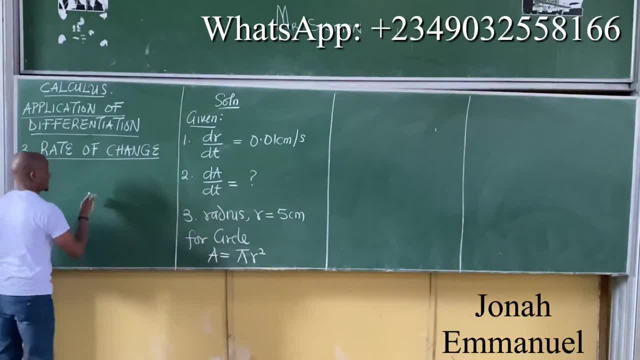 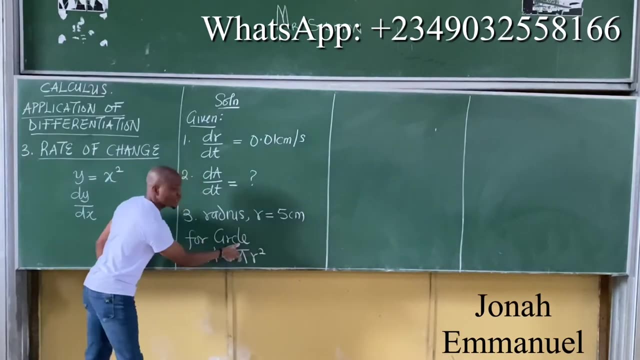 Let me explain something. This is 5, look up see If I have y equal to x square. please watch this: if I differentiate y with respect to x, it becomes dy all over dx. Now here's what you need to know here. in this case, pi is a constant, so as I only differentiate, 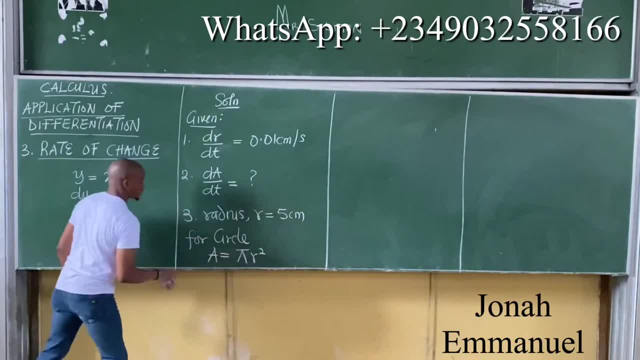 a with respect to what there. If I differentiate this, I should get what there? The A over there, the R Of Z. I'm asked to find the A over the T, not the A over the R. So the question is this: 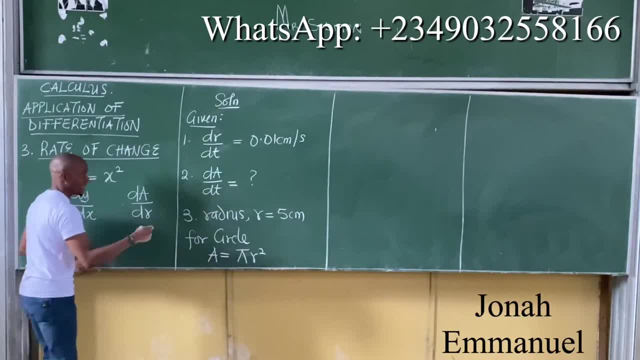 If I have the A over the R, how do I get the A over the T? Now look at this. We can have that, the A over the T. I only have the A over the R. That's the A over the R. 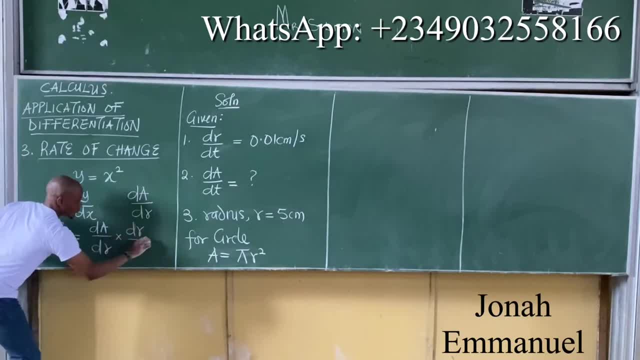 If only I can multiply this by what there? The R over the T, Such that this cancels this. You know what got there? The A over the T, That's it. So from here now, let's get the A over the R. 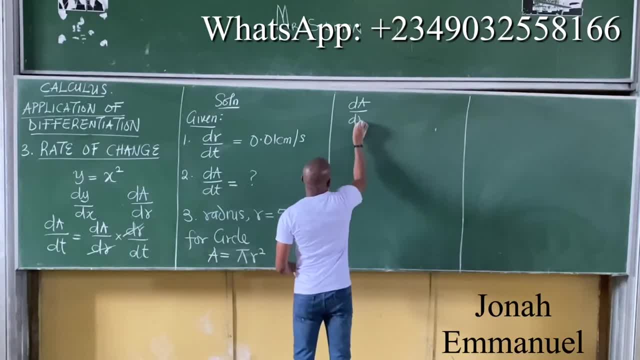 From here I have that the A all over the R is equal to what. What did you get there? 2 pi 1 R, Is that okay? So this one comes down there: 2 pi R. 2 minus 1 is 1.. 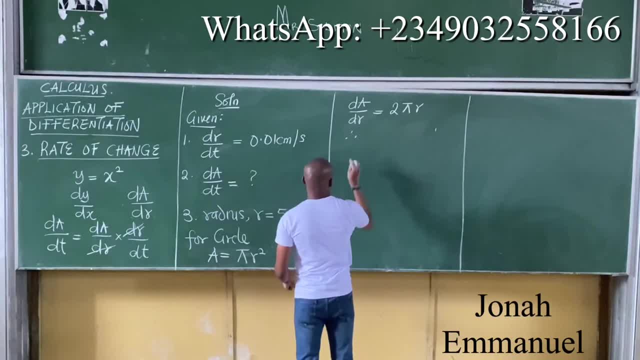 That's 2 pi R. Alright. So therefore, the A all over The T is equal to the A over the R times the R over what there The T? These two cancels out. You have the A over the T. 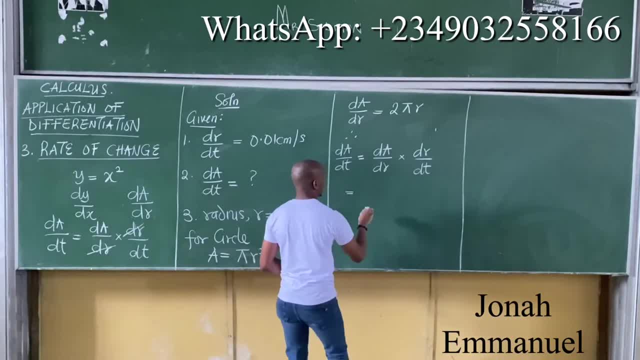 So that's equal to What's the A over the R, 2 pi R times. What's the R over the T, 0.01.. Now I'll tell you something again. The R over the T is in what there. 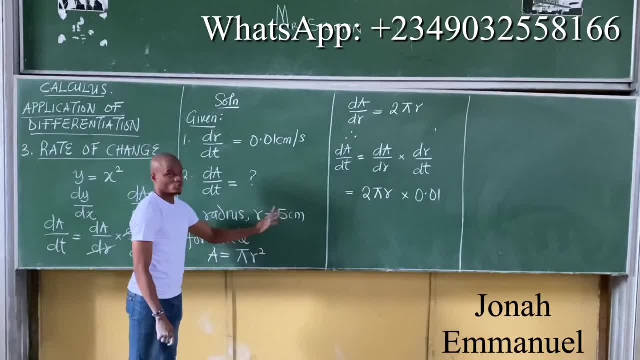 Cm, This one here. There's a word there, Cm, so no conversion. So assuming here was Cm, here was m, I would do conversion. But Cm, Cm, no conversion. That means the A over the T is equal to R. 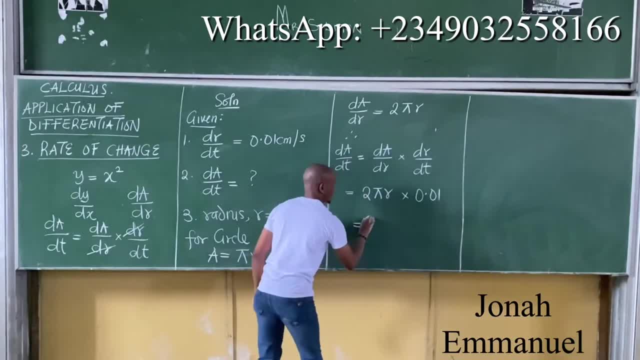 You all know what R is. Yes, Yeah. So what do you got of R? Yeah, We found 2 pi into what's R there, 5 times 0.01.. So here it's equal to this and this: Do you see what's there? 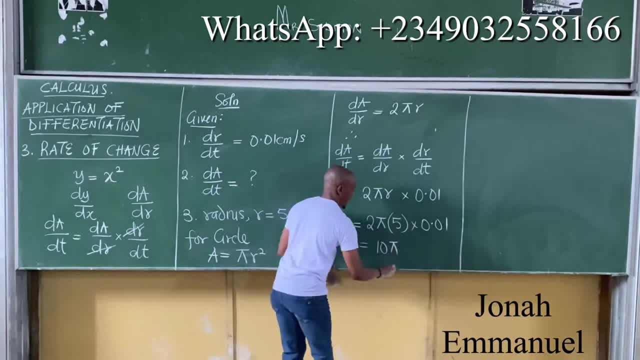 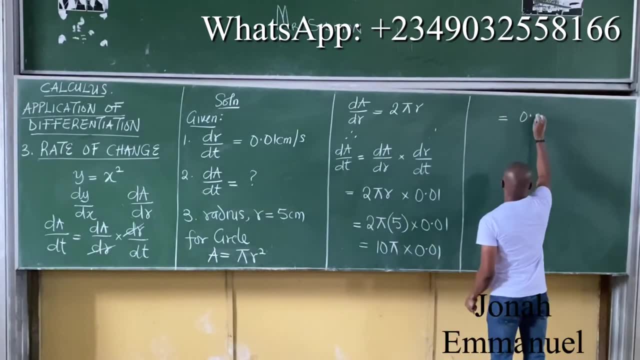 10 pi 2 times 5, 10.. Times 5 times 0.01.. What is that? This is equal to what there? 0.15.. Correct: Yes, If it's 0.15, that's what there. 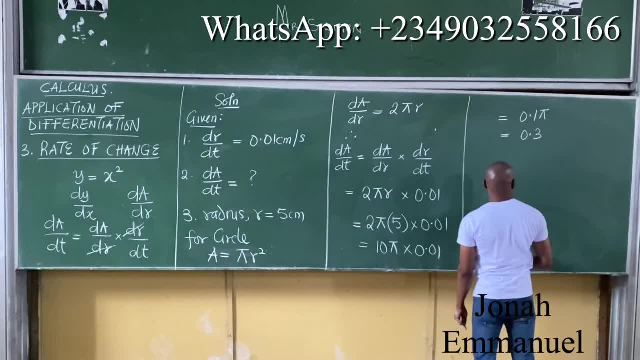 0.. 0 for what? 3, 1, 4, 2.. All right, This is the A over the T: 0.3, 1, 4, 2.. What's your unit? What's your unit? 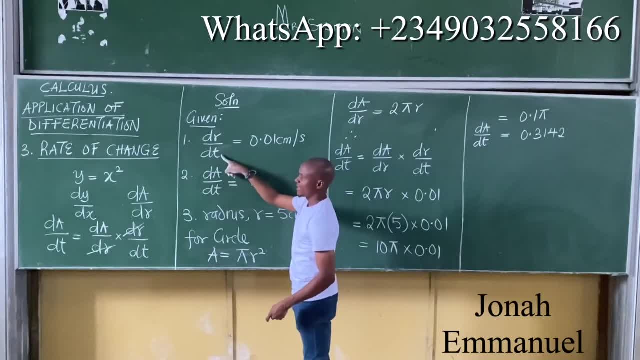 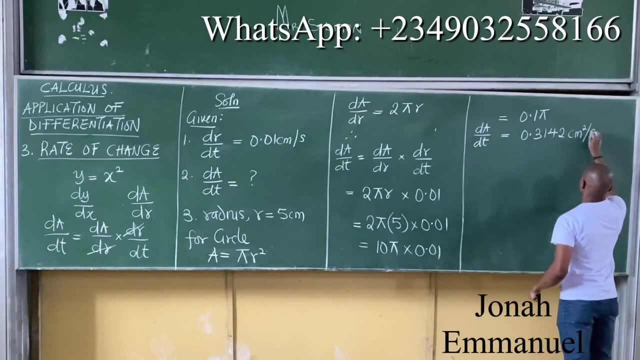 Radius in Cm all over time. in second, Please A, there will be what Cm squared, Cm squared all over time. So this becomes my heartbeat: 0.3,, 1,, 4,, 2 Cm squared per second. 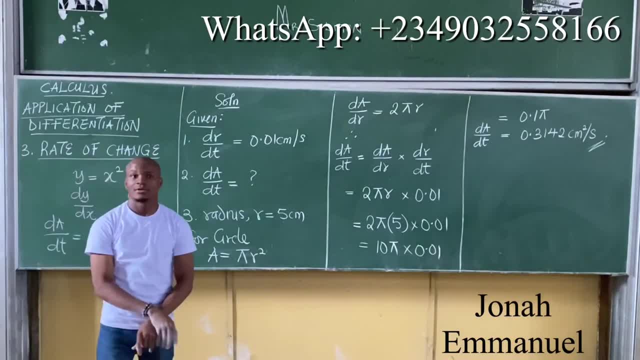 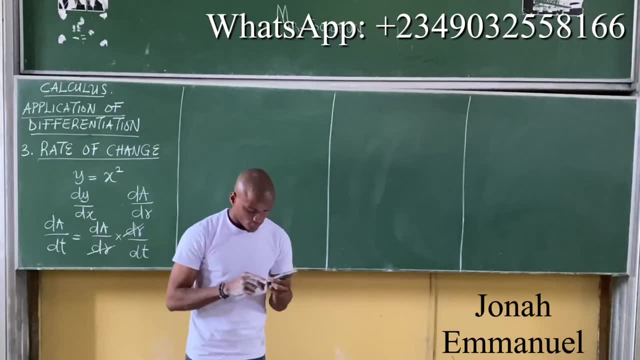 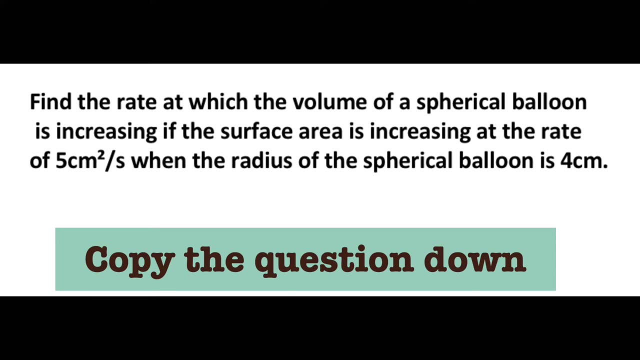 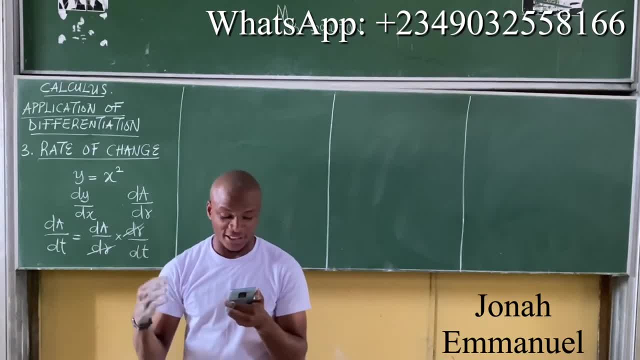 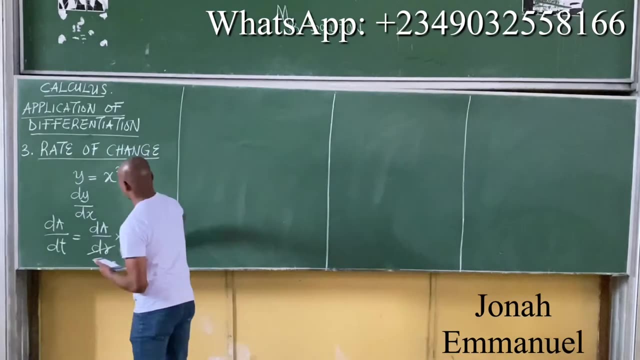 Find the rate at which the volume of a spherical balloon is increasing in the surface area is increasing at the rate of 5 cm squared per second when the radius of the spherical balloon is 4 cm. is 4 cm? First things first, please. First things first please. Solution list out, given parameters, please. 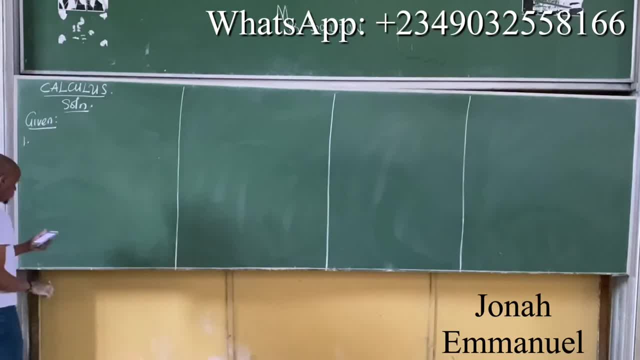 What and what am I given? What's the first you're given there? Hold on, hold on. The first thing is you find something. Find what? The radius of the spherical balloon. So what would it be? The radius of the spherical balloon, The radius and width of the spherical balloon, What would it be? 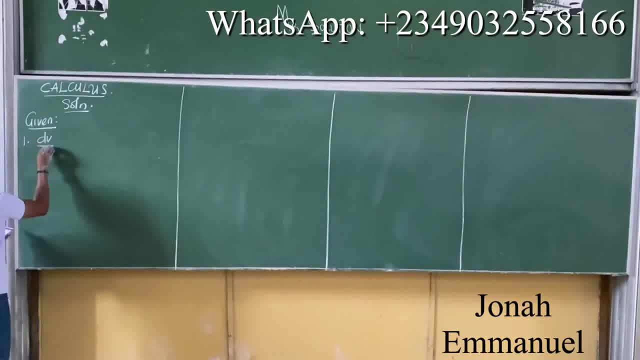 The radius and width of the spherical balloon Right. So I'm asked to find: the ddT is equal to unknown. Okay, Next thing to say: if the surface area is what Increasing, Please, what would that be? The ddT? The ddT is equal to how many there? 5 cm squared per second. 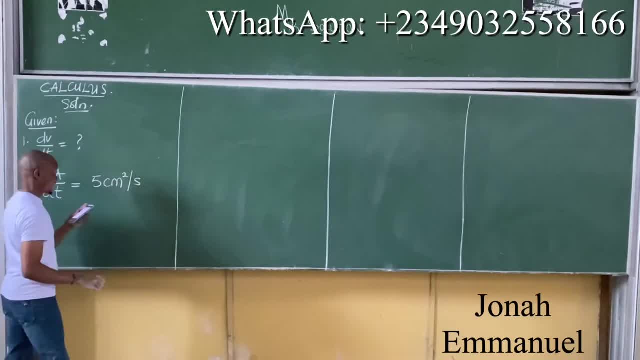 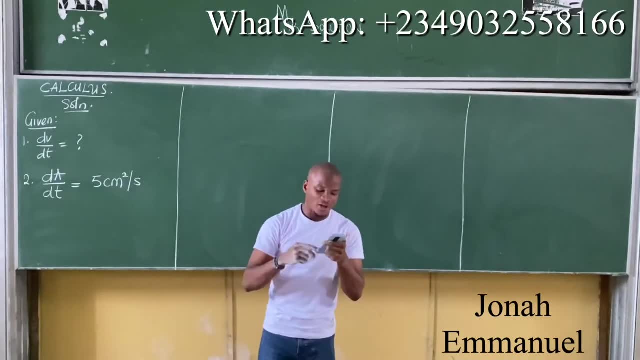 5 cm squared per second. 5 cm squared per second. The z is increasing. Observe, the value is positive, It's increasing. Next thing, to say what and when do you want radius? Number 3, I'm given radius, and how many? 4 cm. 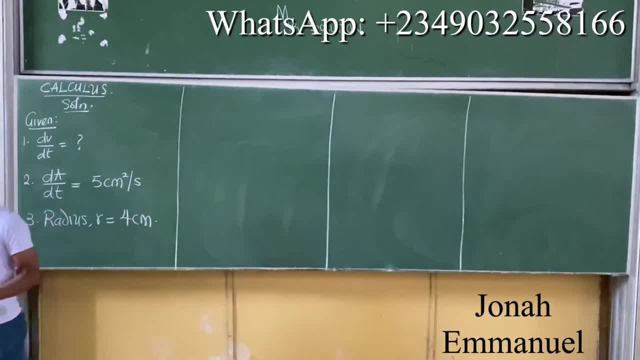 4 cm. Alright, I always advise that, in order to solve the equation, the first thing to do is just analyze it at the reverse part, At the reverse part, At the reverse part of your answer sheet. Do your analysis first. It gives you a focus on what you do first. 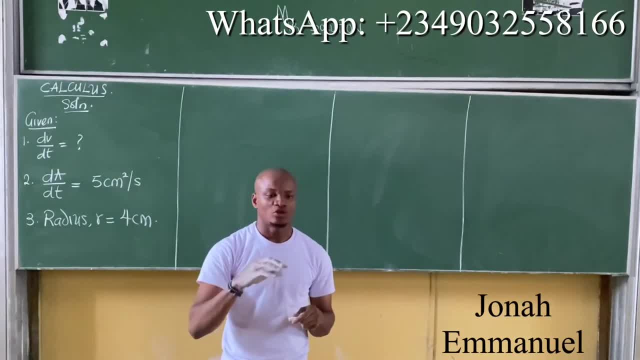 Most of the time, even if you've had this experience, you're trying to solve something and you just end up solving. At the point you just felt like you know what. I should have done this one first. I should have done this one first. 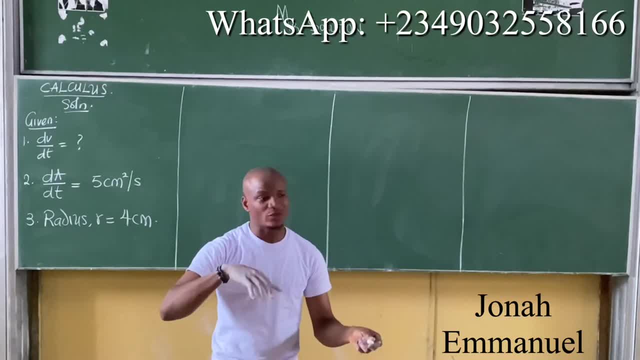 Before this one. You're not sure where to start from where to end. How you go about that challenge is that: do a rough work of what you're about to do. It will guide you. Now, what do I mean In this question? you have to find the VDT. 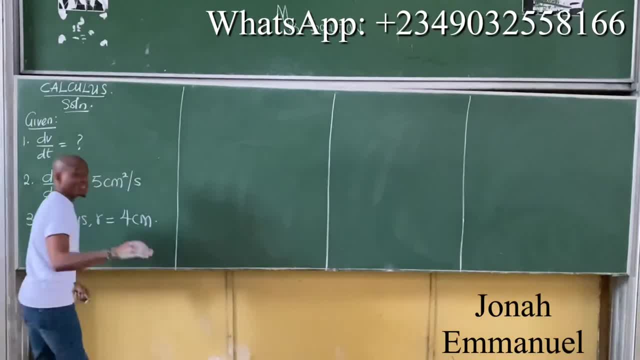 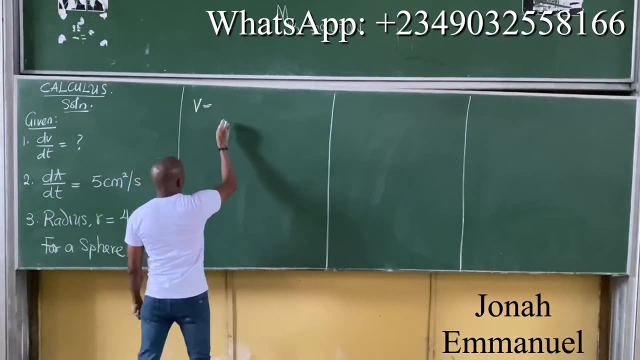 Now first express: which shape is that Square? Alright, so for a square. For a square. they said volume, They said area. What's the volume of a square V? What's the volume of a square there? 4 over 3.. 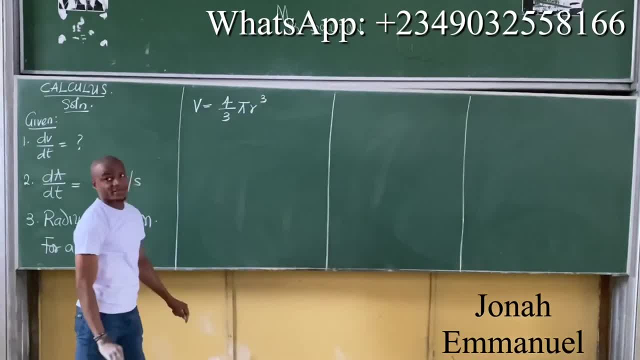 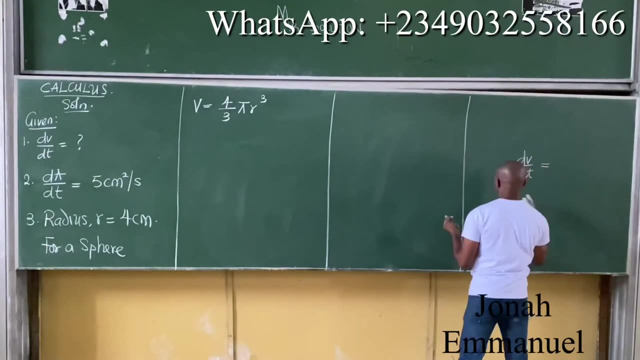 5 over Q, Q, Q. That's volume of a square. Look at this. Here's what we know. We're asked to find the VDT. We know that the V all over the T should be equal to what Observe that V. look at this. 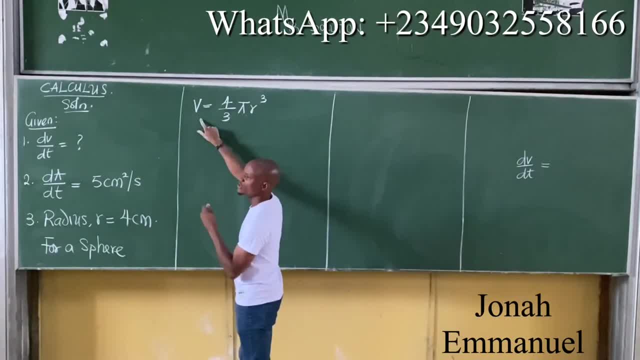 These two are constants. V can only change with respect to what there R, So I can get this as being equal to what there The V over what The R. Can you do what there The R over the T? I can get this value. 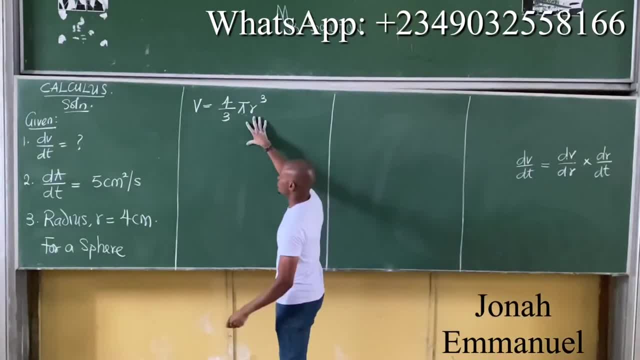 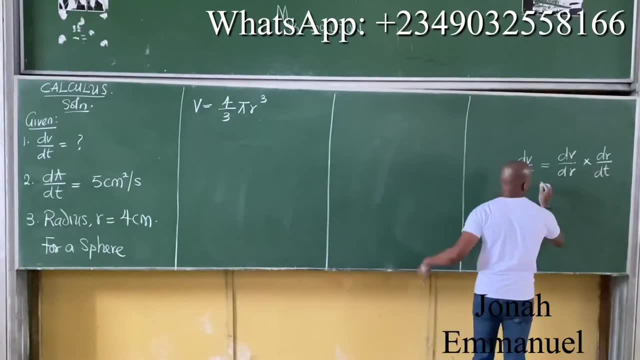 If I differentiate this, I'll get the V over the R. Put the value of R here, So this one is set to. If I have to find the V over the T there, from what I have there, I can get this one. 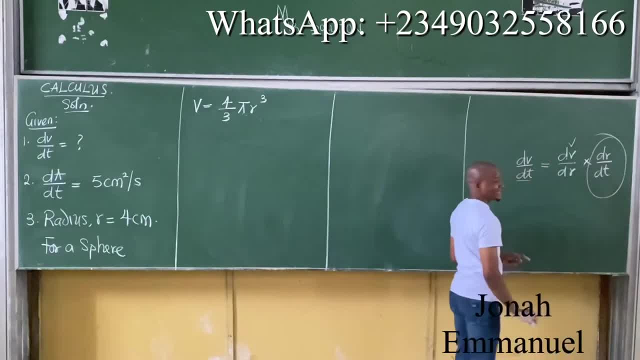 No problem. But then I'm not giving a value of the R over the T. It's not given there. What I'm giving is what The V over the T, Not the R over the T. So my task now would be: how do I find the R over the T? 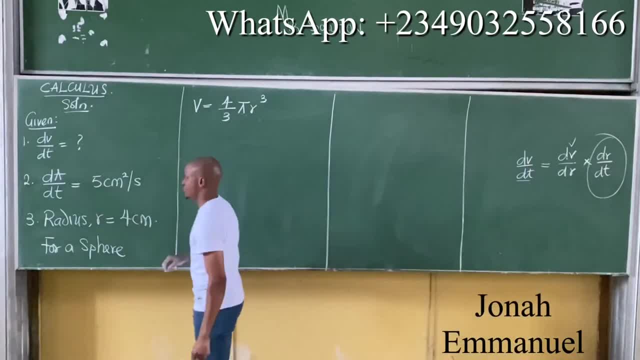 Next up. pick up this one here: the A over the T, That becomes area For the same shape for a square. what area of the square there? Huh, You don't understand what I'm telling you. 4 pi r squared. 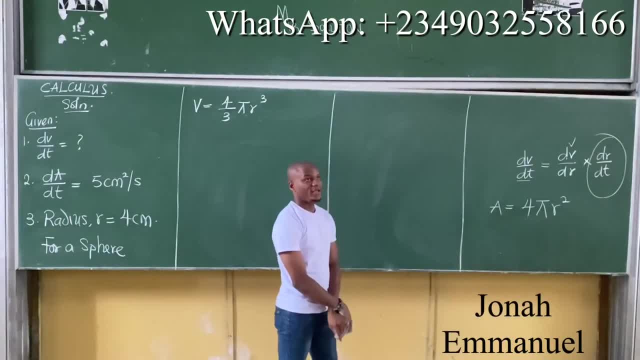 That's the area of a square: 4 pi r squared. Look at this. Look at this. If I differentiate this, I'll get what there The A over what The R. Now check this out From here. that means I can get that. 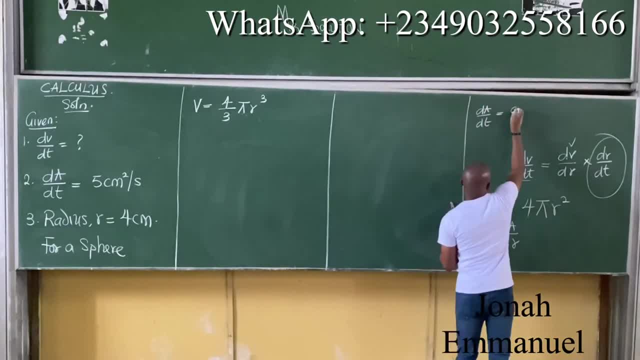 the A all over the T is equal to what there The A over what The R times what there The R over the T. If I do this one here, if I solve this, I can get a value here. So that means I can get a value for this. 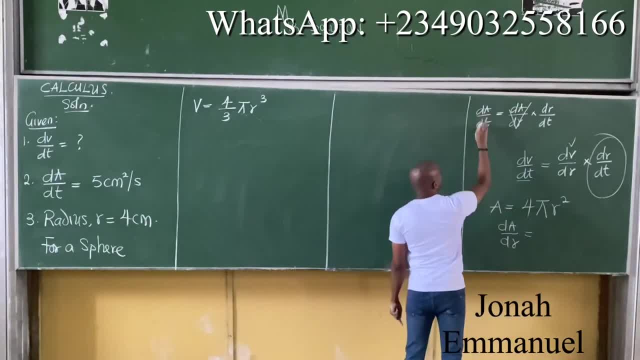 Check. If I look at the board there I'm giving a value for what? A value here and a value here. I can now get this one here, Just divide. So if I divide the R over the T, the R over the T, bring this here. 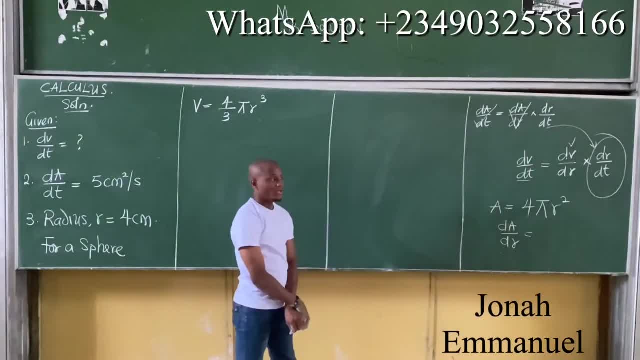 and you've solved the question. That's it. You've solved the question. That's it. By the way, look at this, Look at this correlation. Look at this. Look at this correlation here. Look at a circle For a circle. 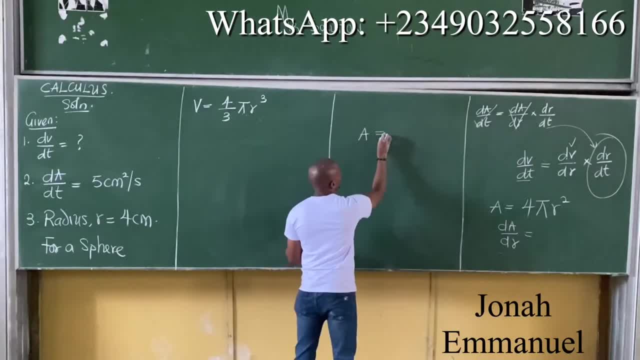 what's your area of a circle? What do you have there? 5 R squared? Please differentiate this. If I differentiate this, what do you have there? 2 pi times R, Please for a circle? what's the circumference? 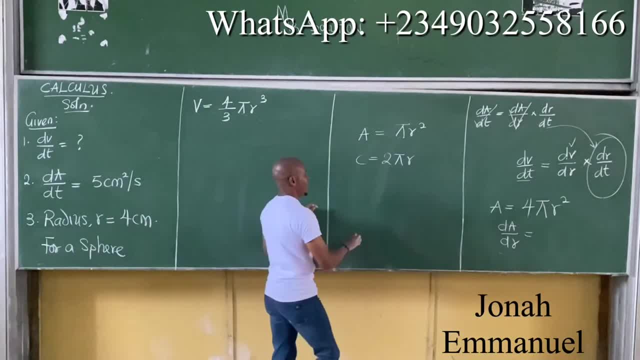 2 pi times R, The same thing. Observe it For a square. what's your volume? This looks like the same thing. When it comes to, when it comes to measurement, I think the biggest one that you can get is volume. 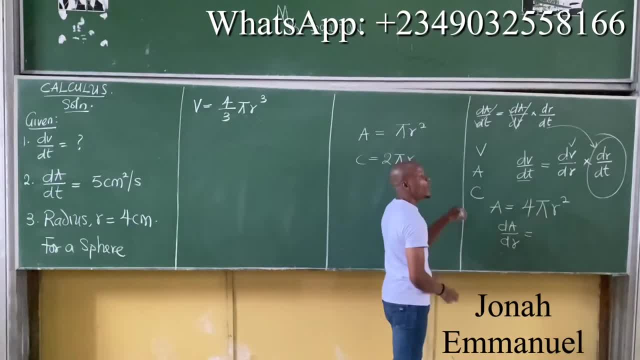 Come down, you get area. Come down, you get circumference. For most input, not all, for most bodies there or most shapes. if I differentiate volume, I'll get area. If I differentiate area, I'll get circumference, As you can see here. 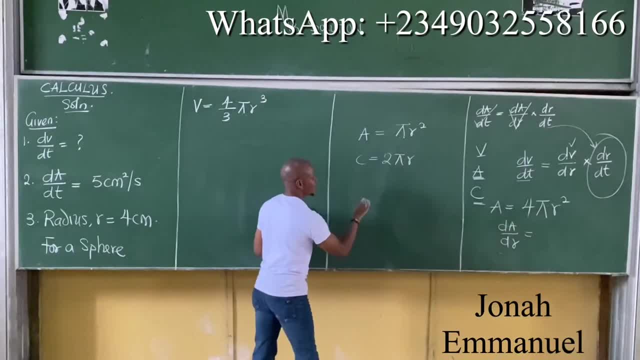 2 for a circle. For a square. we said volume for a square is what V is equal to 4 over 3. pi and Q Differentiate, this V will be equal to multiplied by 3, 3 times 4 over 3. 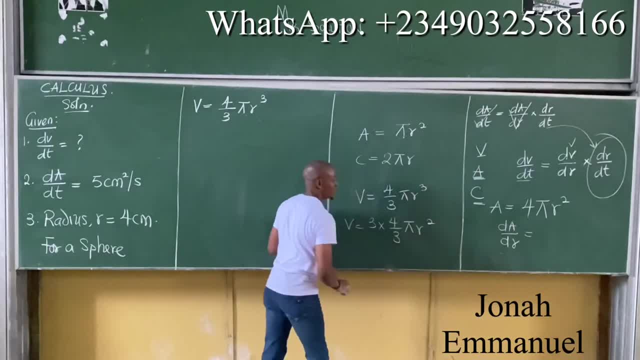 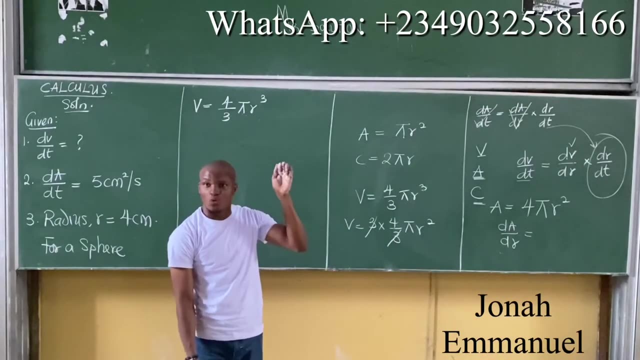 pi and subtract 1, there it becomes square. This stands to go down there and that's the area of the square. It works. You can't look for those shapes where if I differentiate volume I'll get area. At that point you have to prime it too. Just know one. 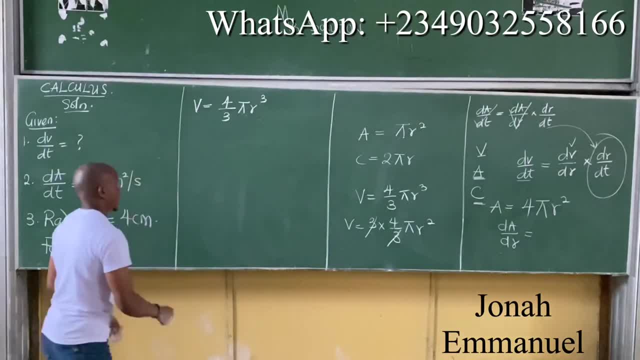 differentiate, you get the other one. It works like that. So first things first, look at this, First things first. from this analysis, from all this stuff here, first things first, let's get, let's start, let's give us volume for now. 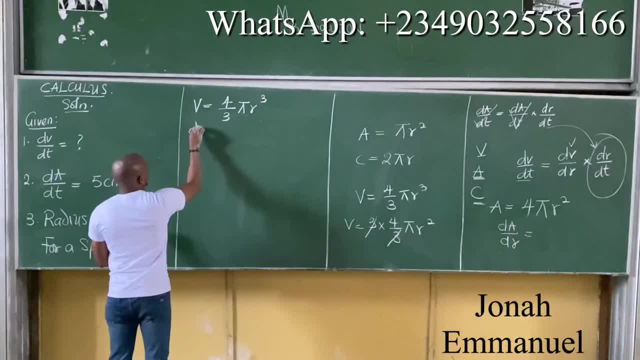 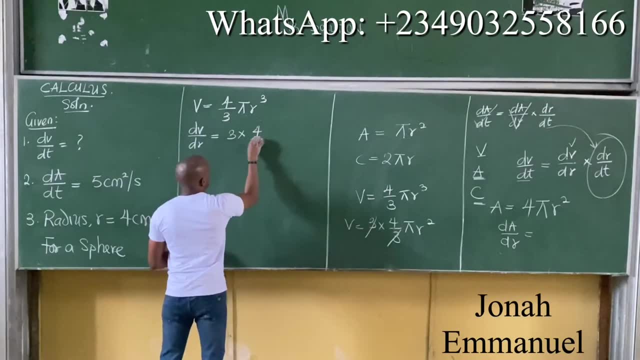 We've gotten V as this: How do you get the V by the r? The V by the r is equal to what do you get here 3 times and differentiate it 4 over 3, pi and Q, Of course, minus 1.. 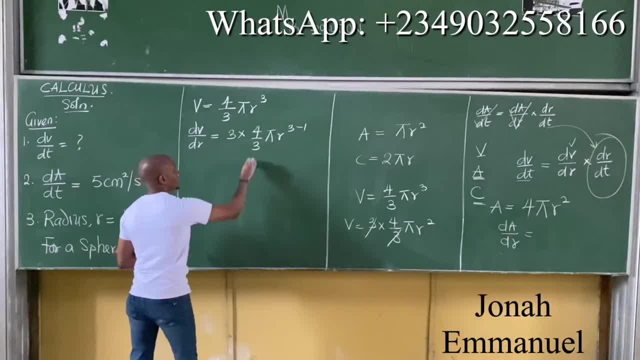 Q minus 1.. Multiply by the power subtract 1.. This cancels this. That's equal to what do you get here? 4 by r squared, This is the V over the r. It happens Next up I have. 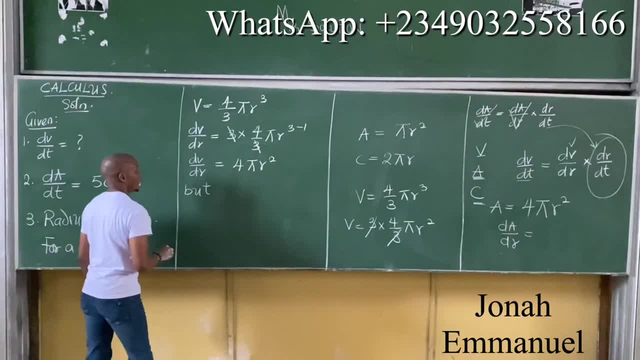 this, But, but also: but. area for a square is equal to 4 pi r squared, That's a. because it's equal to this. Differentiate these two, I'll have that the a over the r is equal to what there. 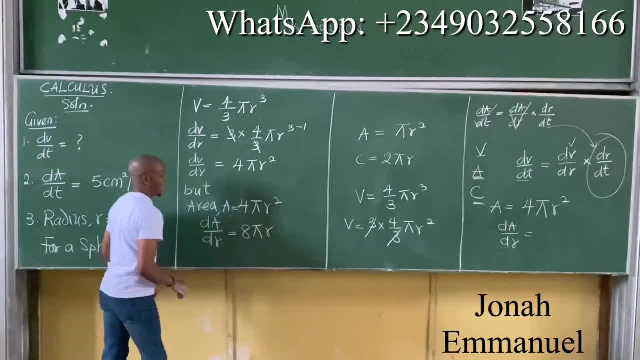 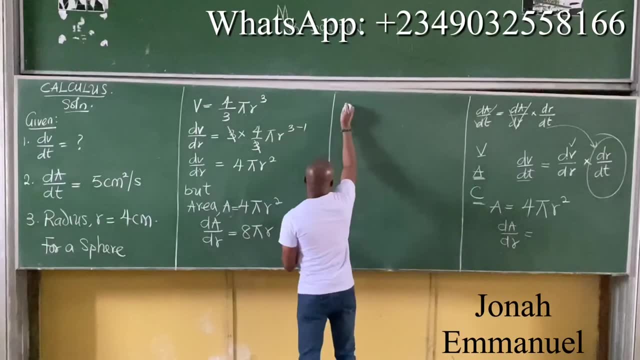 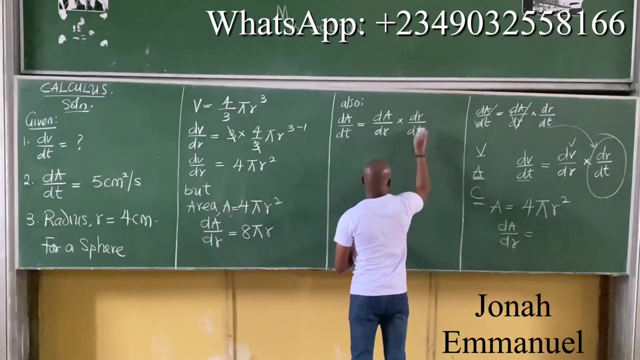 8 pi r, So 8. 2 times 4.. So also we know that the a over the r, the t is equal to the a over the r times, the r over what there, The t? What's? 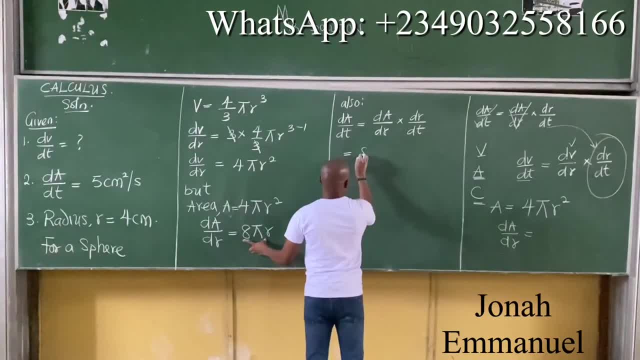 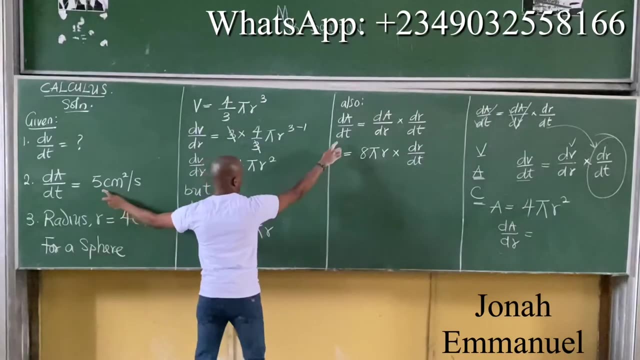 the a over the r. This one here, 8 pi r times. What's the r over the t? Oh no, So the r over the t, But then we have this variable as what there? 5.. So this one here is: 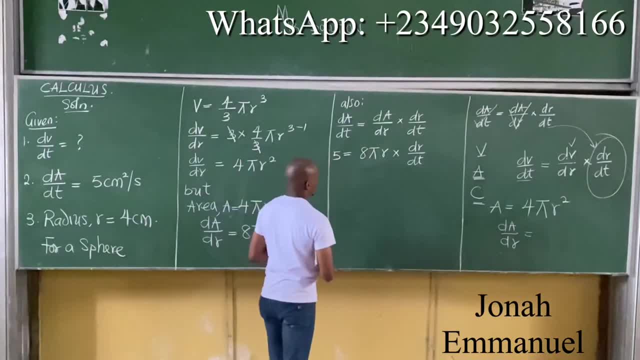 5.. So I have 5 here. Okay, So I have that. 5 is equal to 8 times 5.. What's r? again Times 4 there, So it becomes 4.. So here's your r. 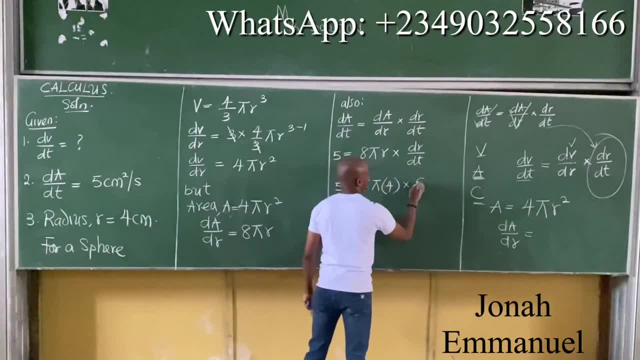 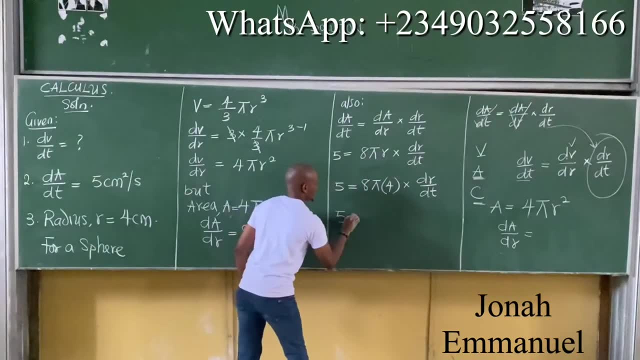 So 8 pi r, That's 4 times the r over the t. Please watch this. Give me like 2 dp, So 5 is equal to Give me this in 2 dp. What do you guys? 8 times. 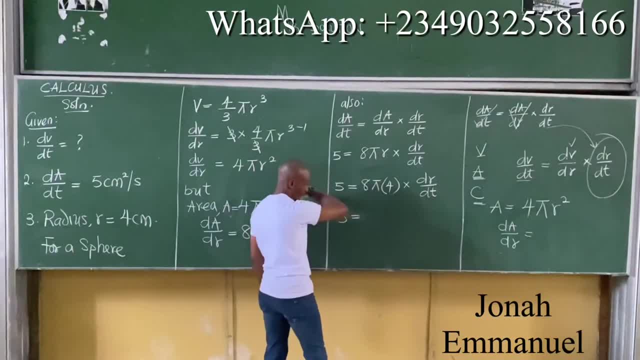 5 times 4 in 2 dp. What do you guys? Right, That's the way we say 4.. What do you guys? 100.. 1, 5, 3.. That's what there, The r over. 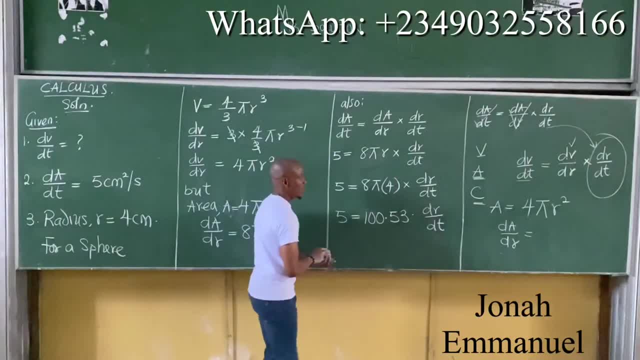 the t. So point is: you get this. So how do you now get the r over the t? What do you do here now? Divide there by what 100.53.. Divide there by 100.53.. So. 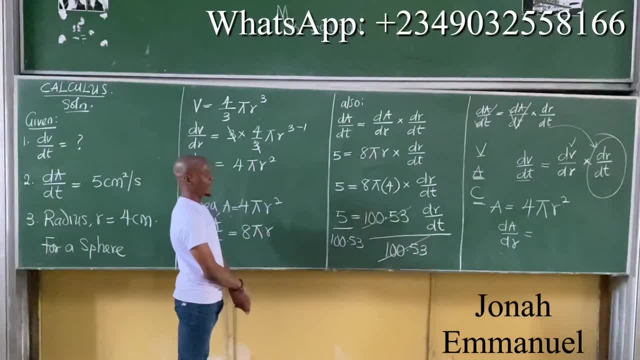 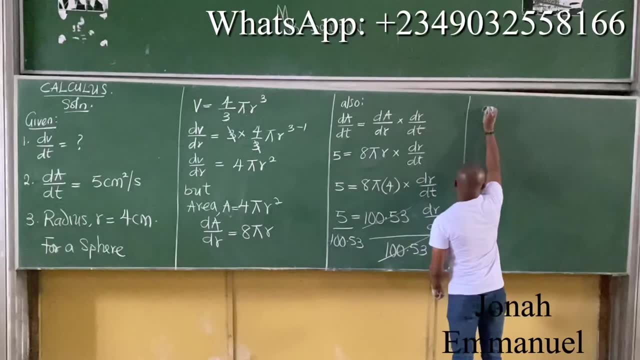 this will now cancel this. I can now get the value for the r over the t. Please give me value. I have that. the r over the t is equal to how many? 0.0497.. 0.0497. 0.0497.. 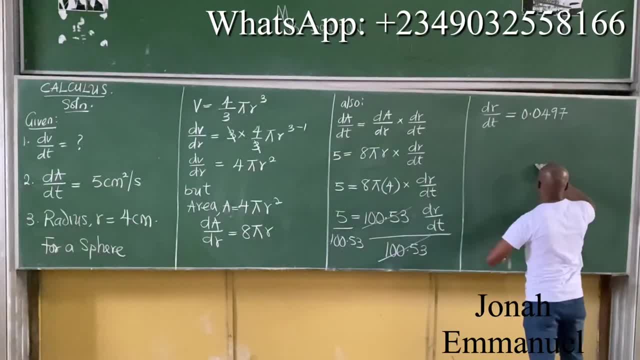 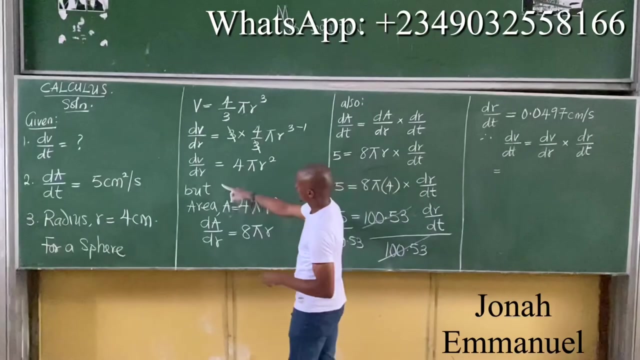 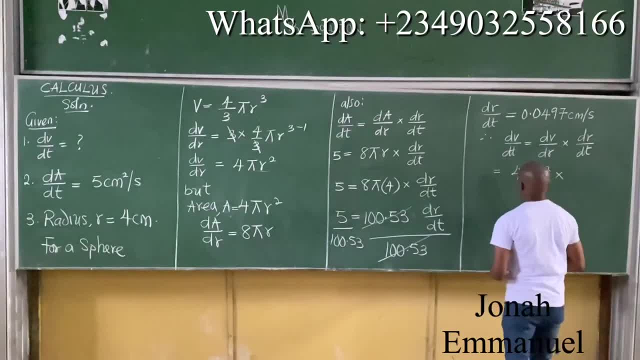 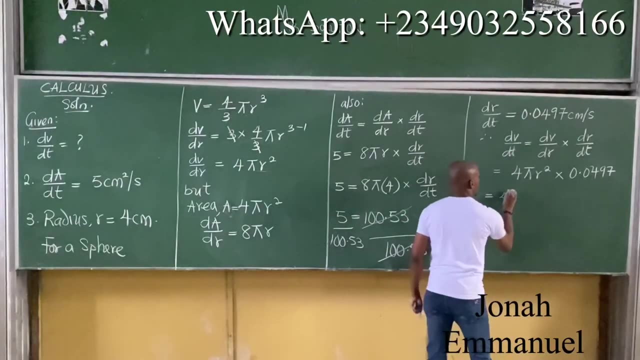 over the R, over r the t. So put the value of r here here, put the value of r here r is 4, so it becomes 4 into pi, into r squared r is 4, it becomes 4 squared times 0.0490.. 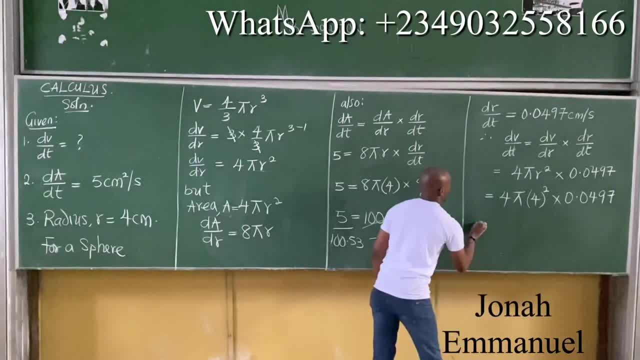 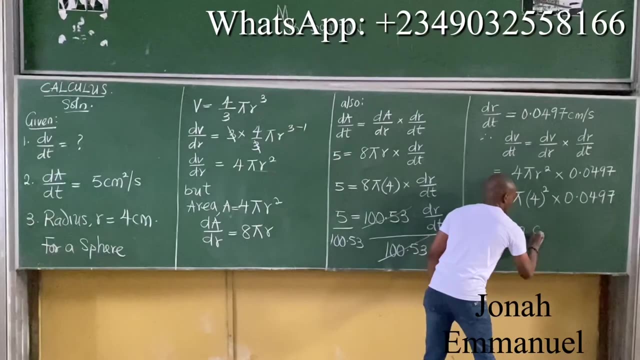 It was worth. like everything. like everything. What do you get? Worth like everything, What do you get? This is 16 times this everything. everything is 9 points, approximately 993 units golden over time. cm cubed per second. 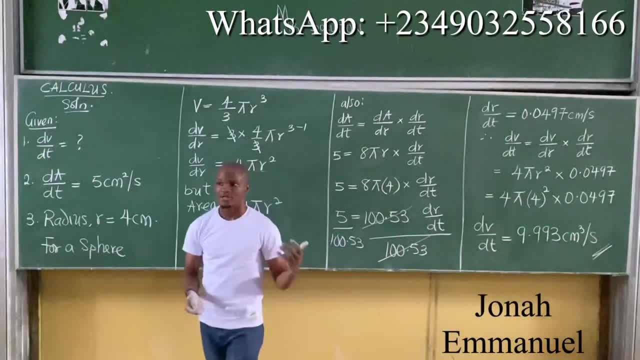 So that's your answer to this: 0 points 993 cm cubed per second. That's how you work out this one, Alright.